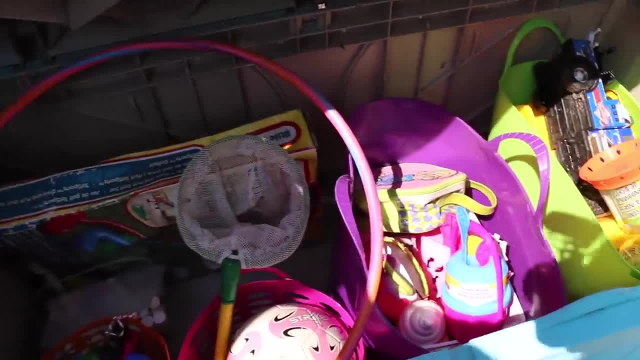 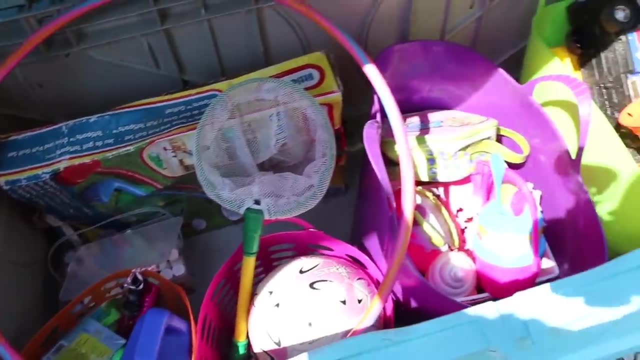 their stuff. I move a lot of indoor toys out every year and it also holds, you know, cars and sporting equipment, bubbles, chalk, all the stuff that kids have sprawled all over the backyard. It's a great place to put it. 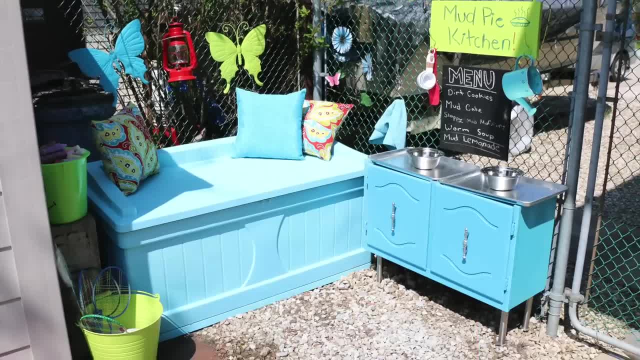 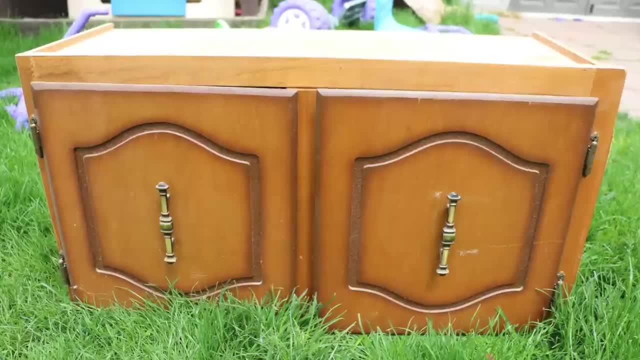 I also wanted to add something else a little special in this space and I saw a mud pie kitchen on Kijiji and I really wanted to make it for my kids. So I had this old cabinet cabinet. We were actually going to donate it or throw it out. We weren't using it anymore. 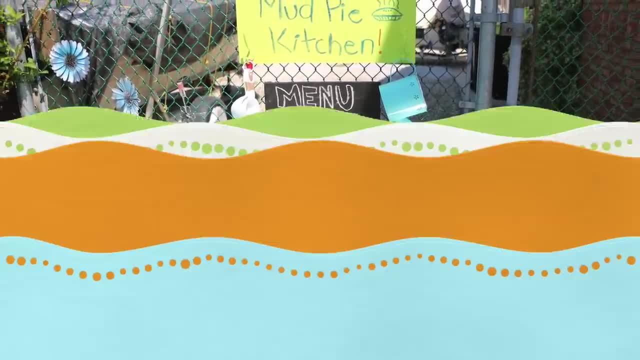 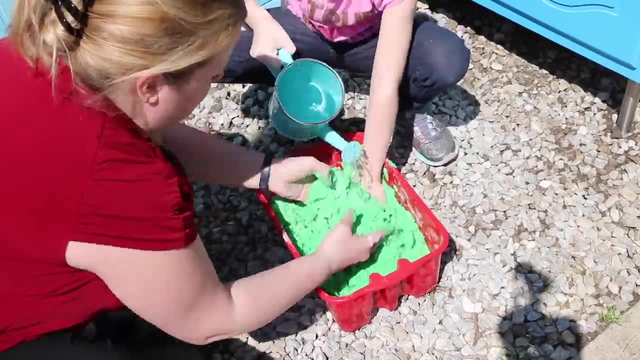 It was a kitchen cabinet, and we transformed it into this outdoor mud pie kitchen. Instead of mud, though, because I'm a freak- we mixed sand, We colored sand, cornstarch and water to make a moon sand. so it doesn't go all over their hands, but they can still really. 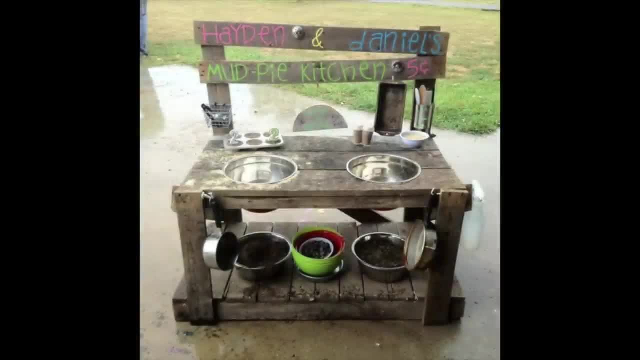 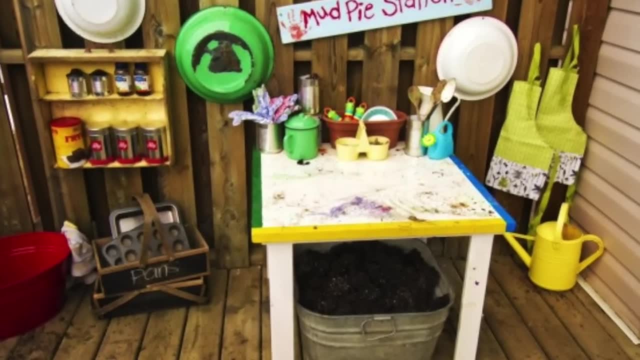 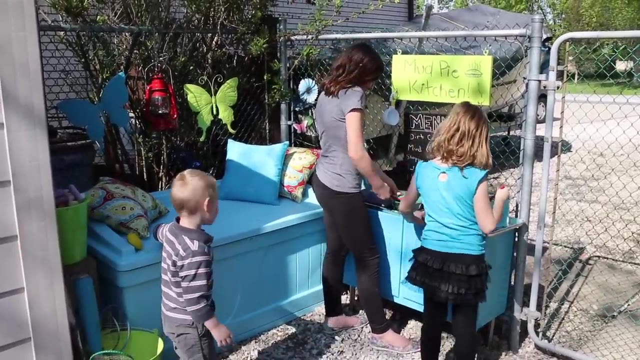 pack it and play with it. I'll add the recipe below. Here's some other examples of some adorable mud pie kitchens. They're using real mud. I'll use moon sand or kinetic sand instead. This was a total hit and the kids played with it for about two hours straight. So if 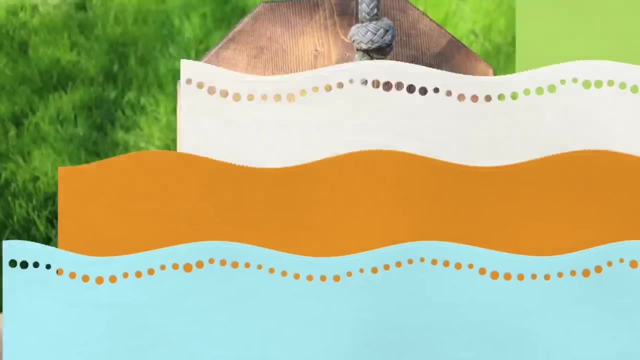 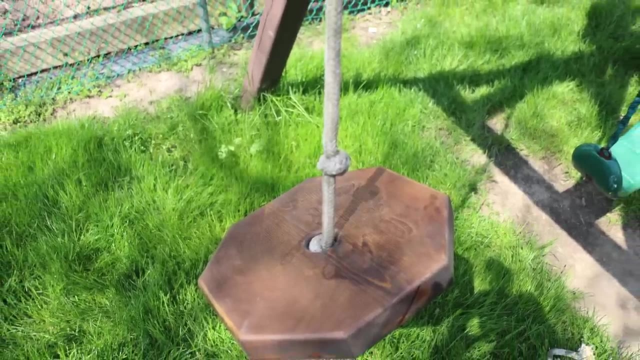 you have kids who complain about being bored, this is a must. The next easy project is this super cool swing you can make in your tree or hang it from your already existing tree fort. I got this idea off Pinterest from livingwellspendingless. 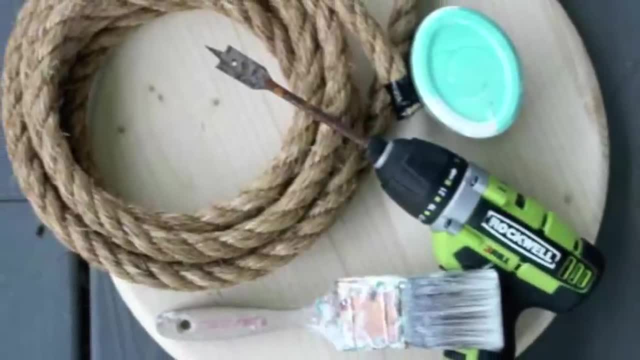 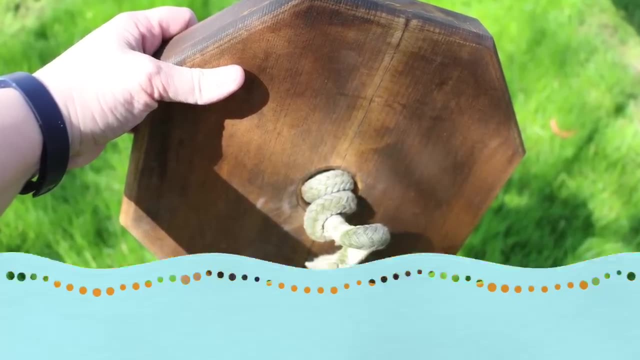 and I mean she spent under five dollars to make this great swing. If you have a tree in your backyard, you can throw this together and your kids will have hours of fun. We already had this piece of wood here. I just drilled a hole in the middle and used the rope that. 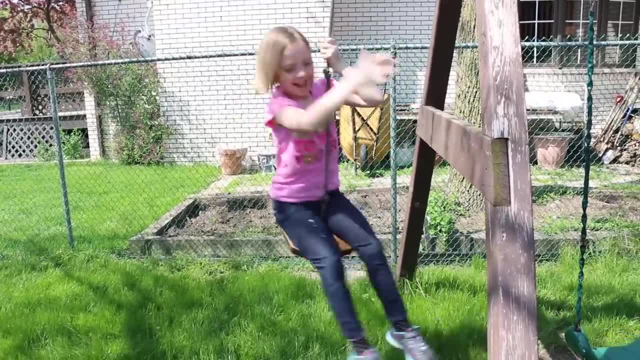 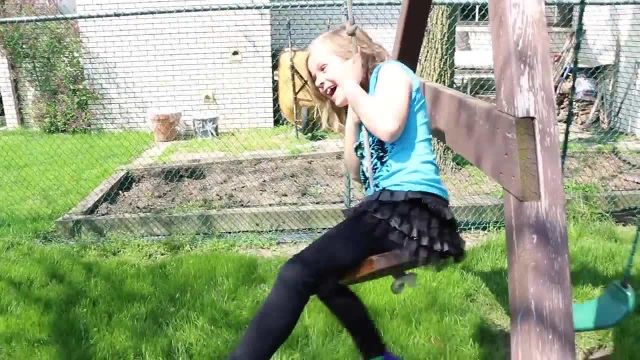 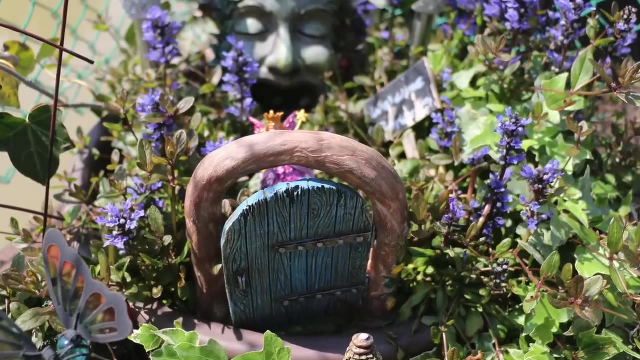 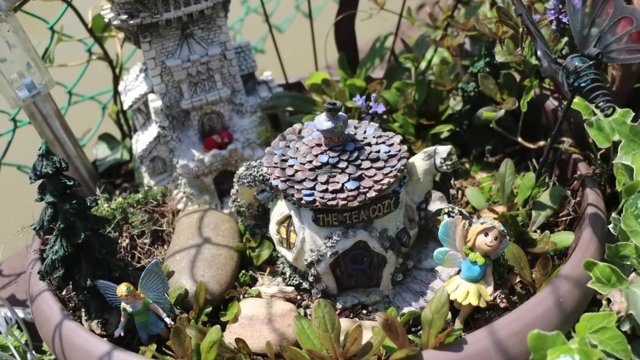 we already had hanging from our tree fort, which was doing nothing to make this super cool swing. The one thing that added hours and hours of fun to our backyard is our fairy garden. We did this last year and all the little things we got were purchased secondhand. You can. 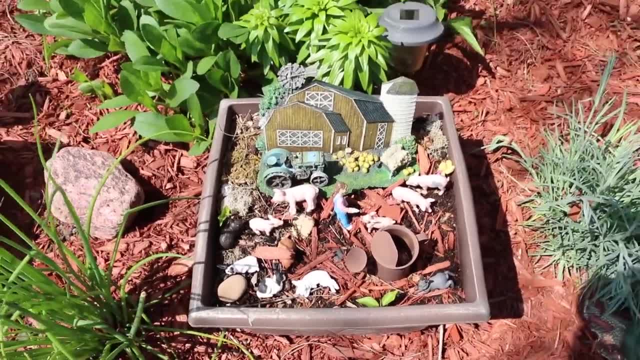 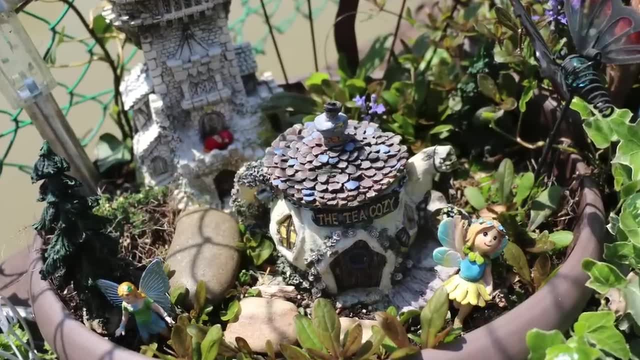 find little houses at Goodwill. You can find them at your thrift shops, Even those old Christmas houses, you know, you can give a quick coat of paint to, or you can do tutorials to make your own. So inexpensive- It doesn't have to be expensive, Most of these things.